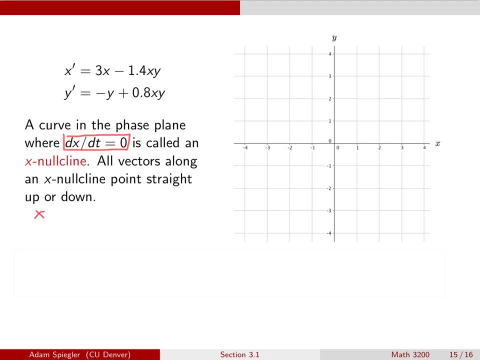 equal to zero. and so if i have this differential equation x prime, i can factor out an x and we see that we have two noc lines. so these noc lines are going to be curves of points, in this case lines. and so we see we have one noc line on the line. x equals zero. and if we were 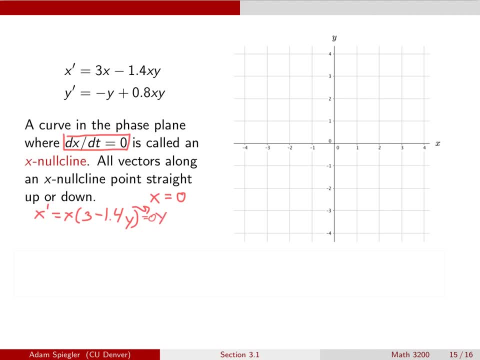 to solve that equation. we would get a second noc line when y is equal to 2.14. so i'm going to plot these lines in the phase plane. so x equals zero, that's the y axis. so i'm just going to put a dashed line over here. 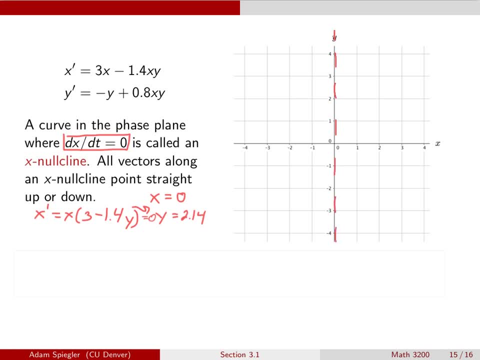 and then the other noc line is through the horizontal line. y is equal to 2.14. so that would be approximately over here, and what we might want to know is: we know that these verticals point straight up or straight down, and whether they point up or down, that really depends. 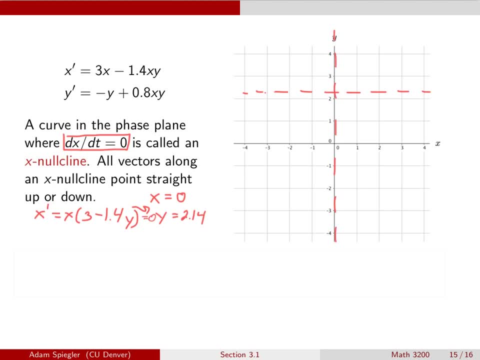 on the y prime equation. so if i were to do some analysis with the sine of y prime, we could say, for example, if x is equal to zero, then this top, then this equation for y prime. that's what i'm interested in seeing is: what's the sine of y prime? y prime is equal to minus pi, and so what we can. 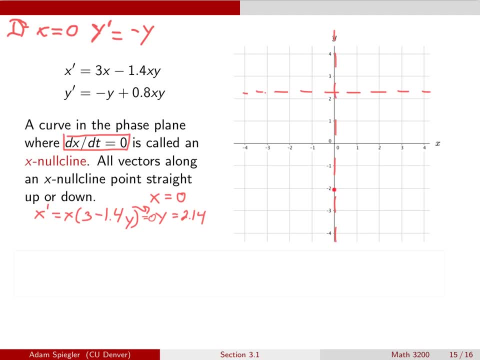 see is if i'm on this line, x equals zero. then what's happening is: if y is negative, then minus y would be positive, right, and that would tell me that y prime is positive. so when y is negative, these vectors are going to point up because dy, dt is positive and on the other hand, when y is positive, then y prime would. 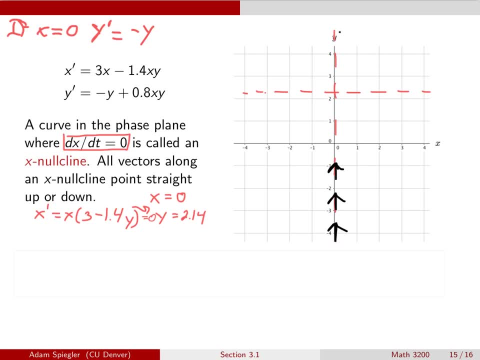 be negative and that's why these vectors are going to point up, and that's why these vectors are going to point down along this x nullcline when y is positive, okay, and so we still have some work in terms of figuring out whether how the vectors are pointing up and down along this other x nullcline. 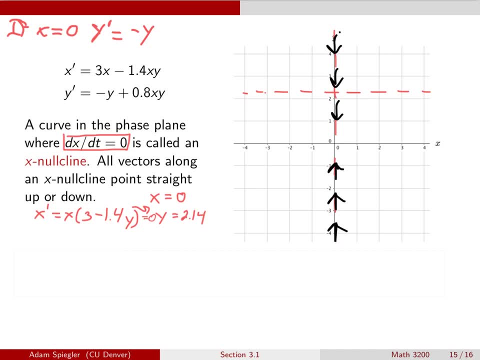 but i'll come back to that in a sec so we can look at a similar idea. we've seen this: that we get important behavior as well at any point in the phase plane when dy, dt is equal to zero. we call these y nullclines and all of the points along these curves are going to 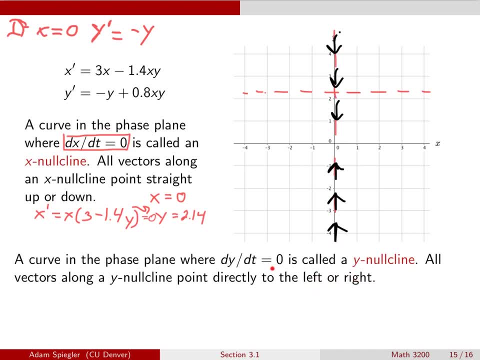 point directly to the left or to the right, because they're going to have no vertical component to those vectors. and so to figure out how to find the y nullclines here it's a similar process, but now we set the equation for dy dt equal to zero, so here we would set y prime. 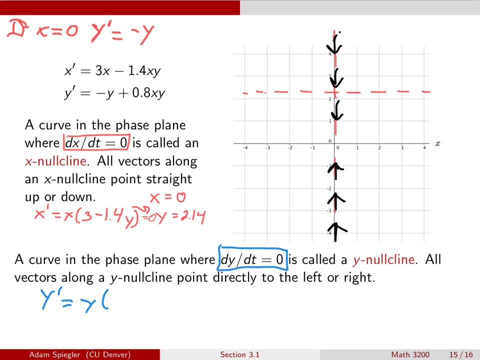 which is we could factor out a y from the equation and when we get minus one plus 0.8 x and we can see that this is equal to zero when y is equal to zero. so that means we have one y nullcline along the x-axis when y is equal to zero and we have a second nullcline when that. 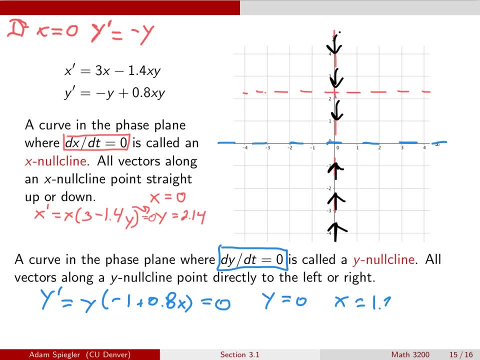 other factor is zero, and that's going to occur when x is 1.25. so we have a second nullcline, y nullcline over here, and then we want to figure out how, whether these vectors, we know they're pointing directly to the left or to the right. but is it to the left or is it to the right? and so 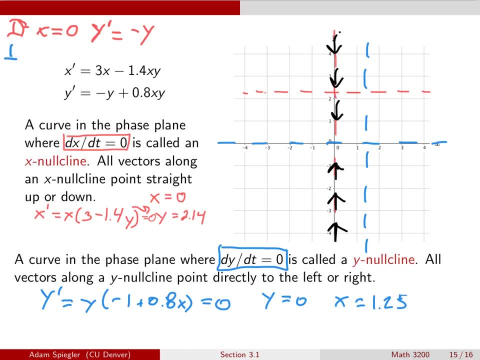 here we can do a similar sort of analysis and we can say: well, if y is equal to zero, so I'm going to consider the nullcline along the x-axis. now we would want to look at what's the sine of x prime, because that's going to determine whether we go to the left or to the right, and so we're going to 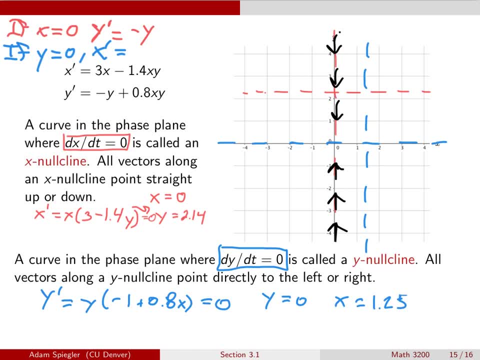 consider the nullcline along the x-axis. now we're going to consider the nullcline along the x-axis or to the right, and so here we can see that x prime. if y is equal to zero, then this term goes away in the differential equation for x, and what's left is x prime is going to equal 3x. 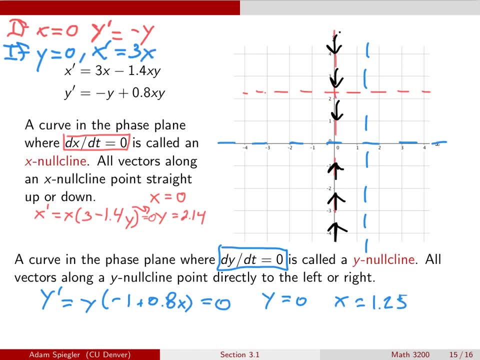 and so we see that if x is bigger than zero, then x prime is going to be bigger than zero. so for all of the points along this curve, as long which is a line, as long as x is positive. so when I'm over here, we see that the vectors are pointing to the right because x prime is positive. so I'm 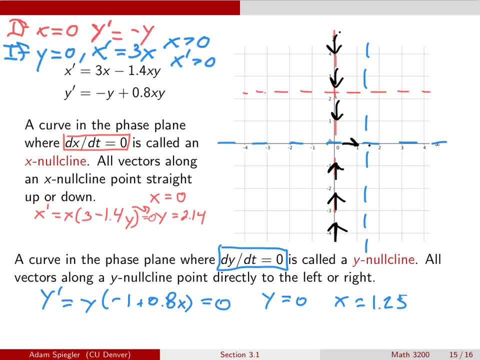 going to plot these vectors over here. they point to the right and same idea. we could identify that these are pointing to the left and I would encourage you guys to think about what to do with the other nullclines. the analysis is the same. maybe the algebra is just slightly more difficult. but what you should be 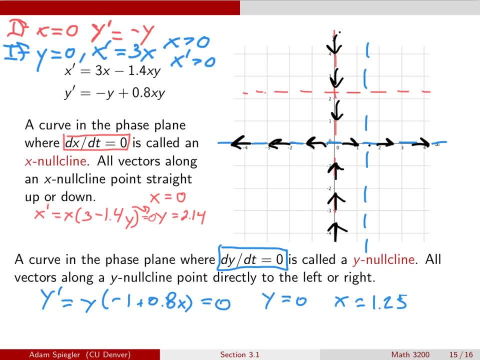 able to show is that along the nullcline for y is equal to 2.14 as long as x is bigger than 1.25, you'll see that in this case y prime is positive and that's why these are pointing up. and when I flip and all of a sudden x is less than 1.25, then these vectors point down and 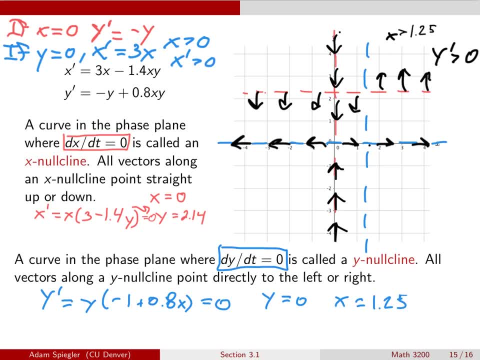 if we were to look, finally, at the nullcline, when x is equal to 1.25 along this vertical line, what you could verify is that in this case, if we set x equals to 1.25, then what we can see is that when y is bigger than 2.14, you should see that x prime is going to be actually negative. 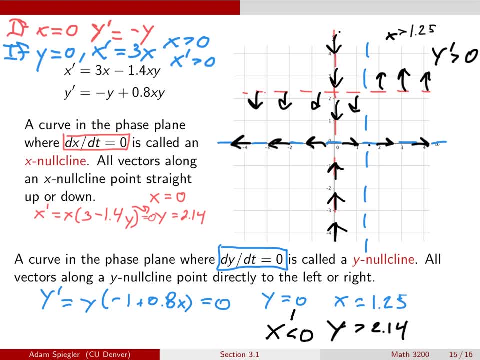 so that means when y is bigger than 2.15, these vectors are actually pointing to the left. so that would mean we've got these vectors pointing to the left and then, when y becomes less than 2.15, x prime becomes positive and now our vectors point to the right and in the